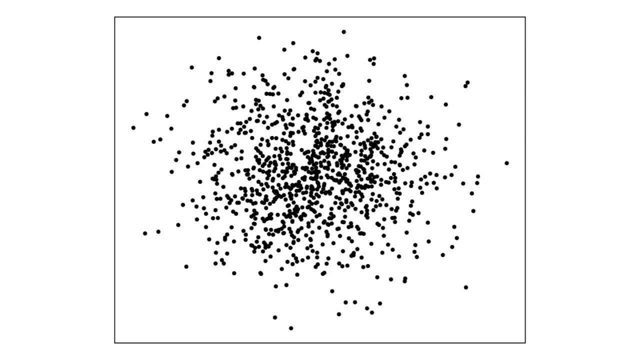 Well, imagine that you have the following data and you want to create a distribution you want to use to sample new data. Although not perfect, a good initial guess would be to say that the distribution of the data points in the cluster of its nearest neighbors is the same as the distribution. 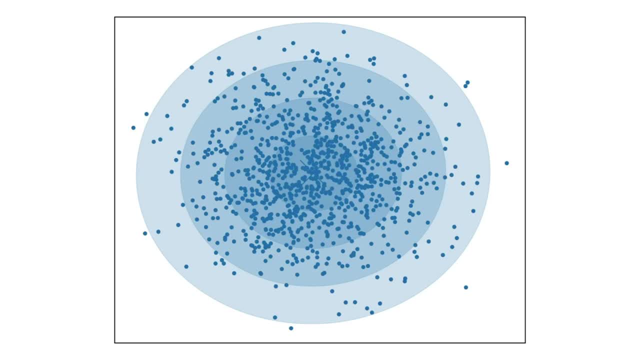 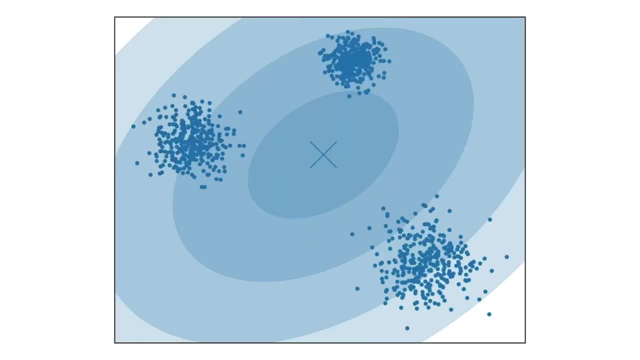 of the data points in the cluster of its nearest neighbors. So let's say that this data comes from a Gaussian distribution and try to fit such a model on top of it by using something like the maximum likelihood estimation. However, what do you do if your data looks like this: Simply fitting a Gaussian distribution. 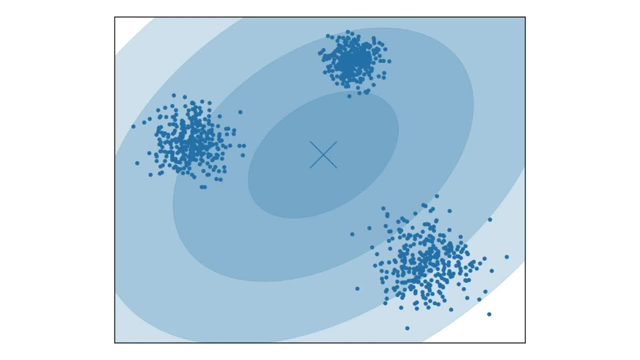 would not yield good results, since this data is grouped into several clusters. So in order to have a much more representative distribution for it, you need to fit a Gaussian on top of each cluster, which is basically what GMM tries to achieve. 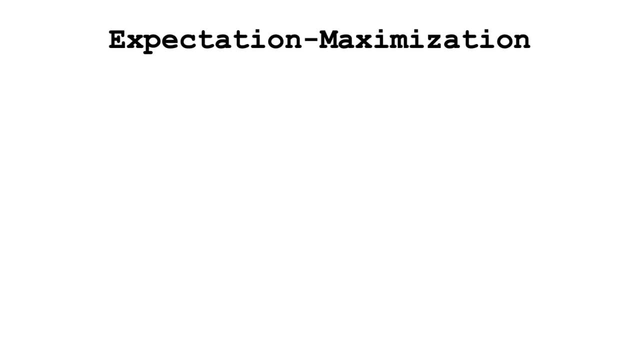 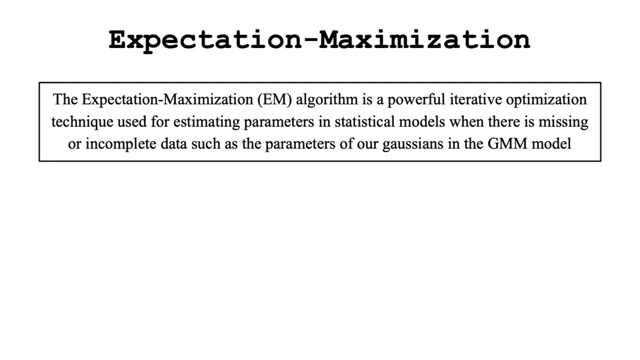 The mathematics behind this is quite simple yet elegant, and the algorithm relies on the Expectation Maximization algorithm to find the best possible fit for our Gaussians. In short, the Expectation Maximization algorithm is a quite powerful iterative optimization method that's supposed to estimate parameters in statistical models when there is missing or 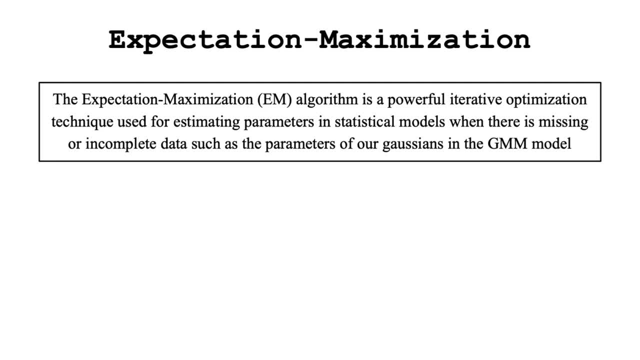 incomplete data, such as the parameters of our Gaussians in the GMM model, And it consists of iteratively applying the Gaussians algorithm to find the best possible fit for our Gaussians. The Expectation Step, where the algorithm calculates the expected value of the log. 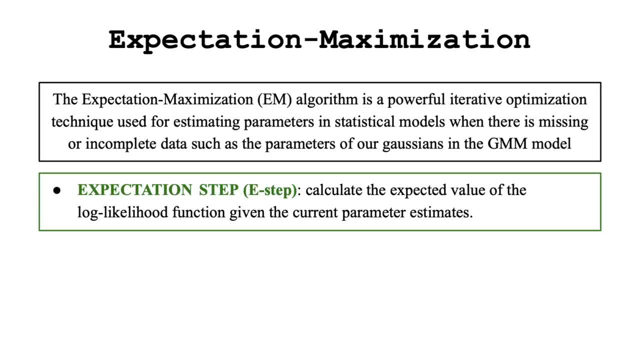 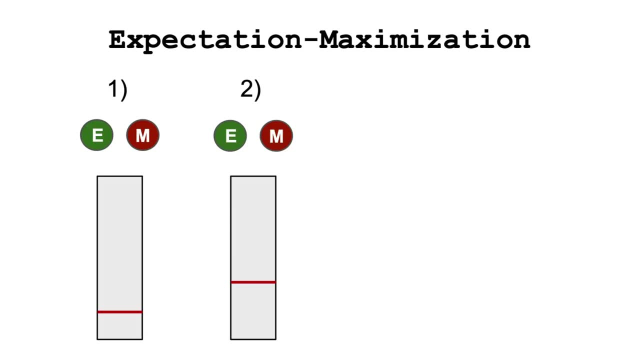 likelihood function given the current parameter estimates and the Maximization Step, where the algorithm updates the parameter estimates to maximize the expected log likelihood calculated in the E-step. So, in other words, what happens is that we are bootstrapping from our initial guess. 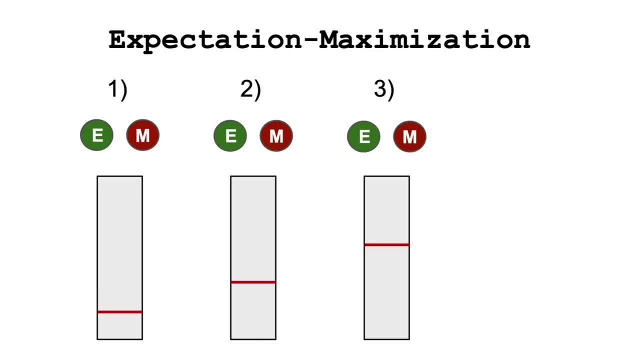 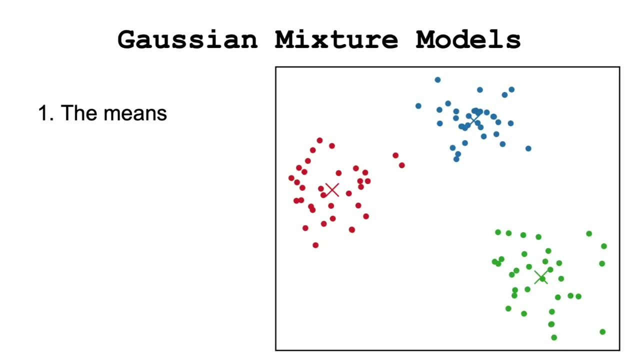 by alternating between the E-step and the M-step, allowing us to find our parameter estimates. For the GMM model, this translates to, firstly, having an initial guess of where each Gaussian should be centered, how their covariance matrix should look like and how much weight we should provide to each Gaussian in the final distribution. 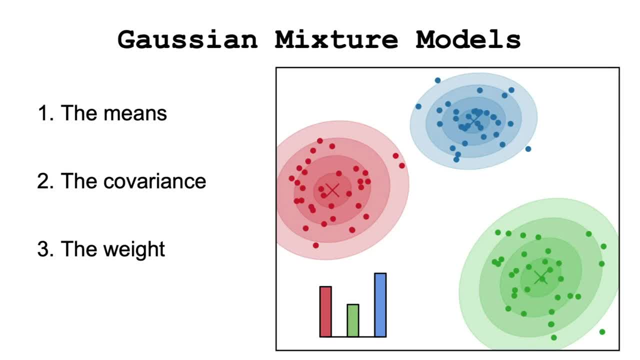 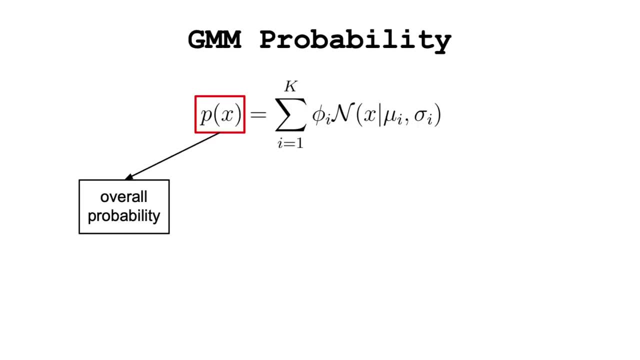 All these are the latent or hidden variables of our model that we don't know and that we are trying to estimate. And now let's look at the mathematics of Gaussian mixture models. Simply put, the probability of sample x is equal to the weighted sum of probability that the sample has in each.